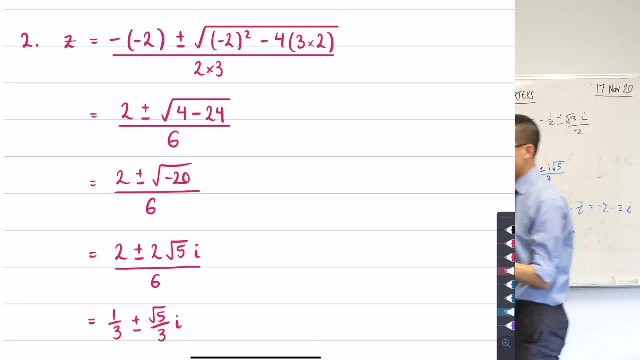 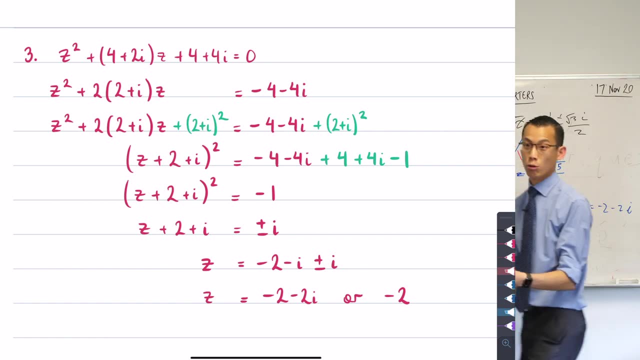 coefficients, And those complex coefficients make a solution, And those complex coefficients make a straightforward use of the quadratic formula. teeny bit, messier. So you may have done that and you would have arrived at the same answer, but this is how my working looks. It's how it looks. 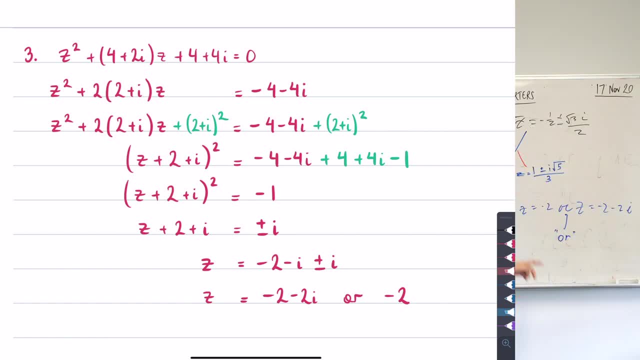 okay, Completing the square you'll arrive at. have we got here? Let's see negative. two minus two minus two. i Looks good to me, right. The advantage is you don't have to deal with long, awkward square root signs and the enormous fraction that is at the heart of the quadratic. 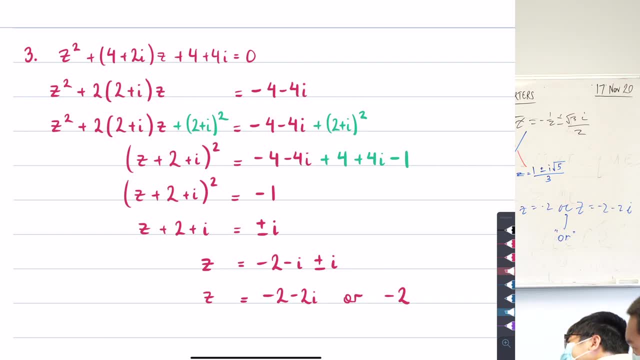 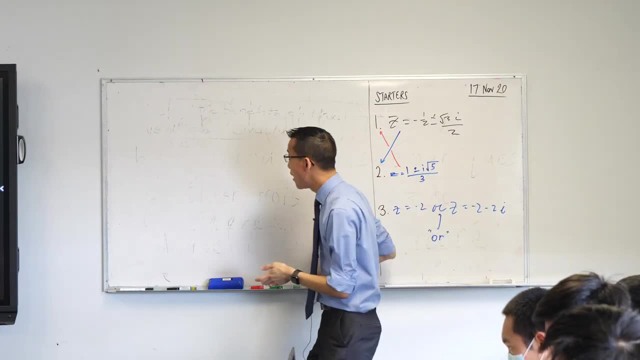 formula, But all of the arithmetic ends up being the same. So whichever you feel best with that's okay with me. Are you happy with that? Thumbs up, Please rule that off. And then the heading I would like you to make is: 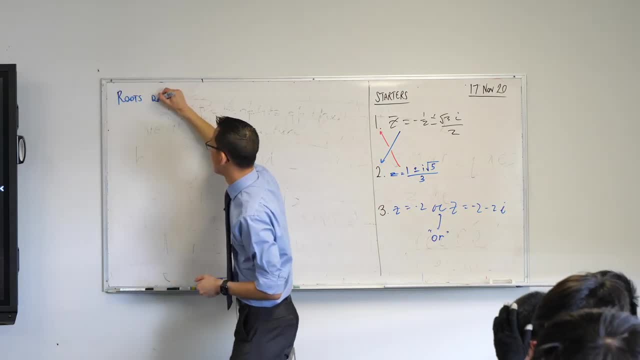 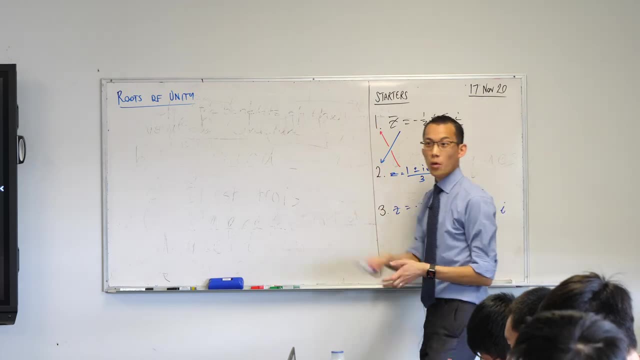 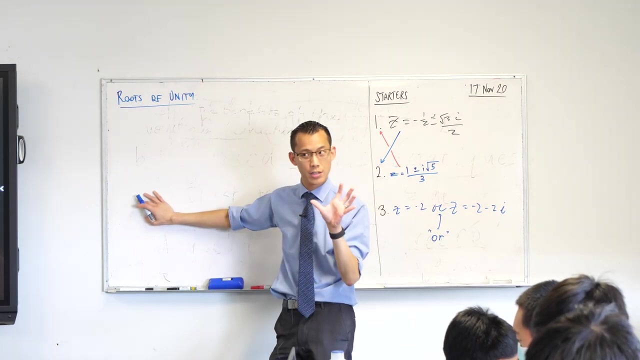 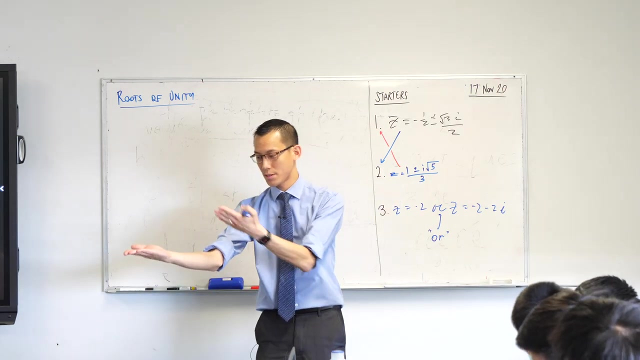 roots of unity. Now let me explain what this means before we dive right in. Last time we were having a look at solving equations that end up with complex solutions like these right Now. one of the reasons for that was so that we could move from square roots of complex numbers. 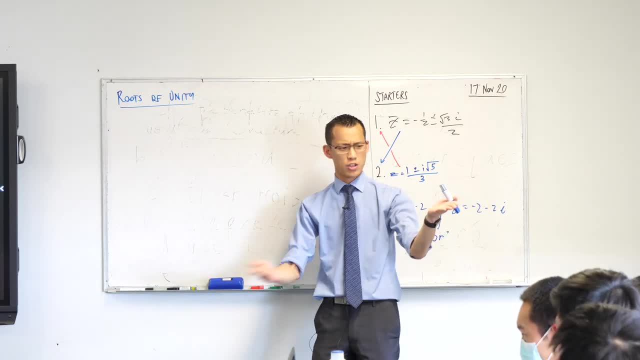 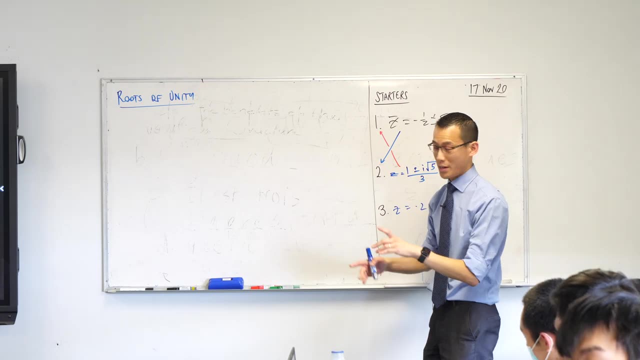 into general roots of complex numbers, Not just square roots but maybe like cube roots, fourth roots, fifth, whatever number. We're going to have a look at nth roots all of this week but in order to make things like sort of ease us into this, we're going to look at the nth roots. 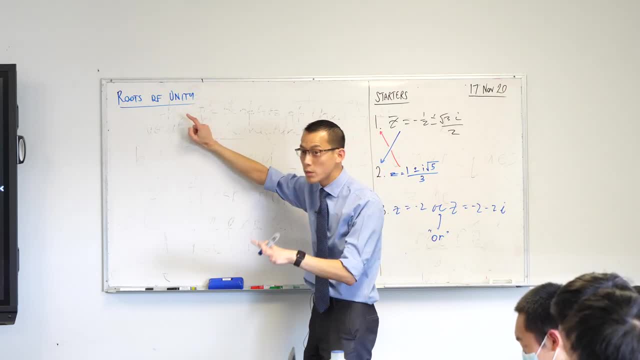 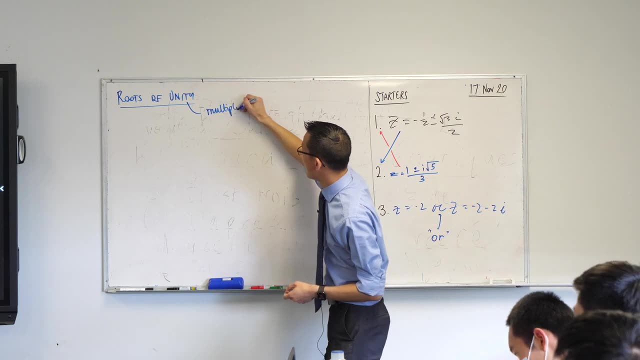 of a particular complex number called unity. Now, this number is really important. It's so important. it doesn't just have a fancy name like unity. It's got another fancy name: It's called the multiplicative. you can write this down because it's kind of- I mean, it's not within the scope. 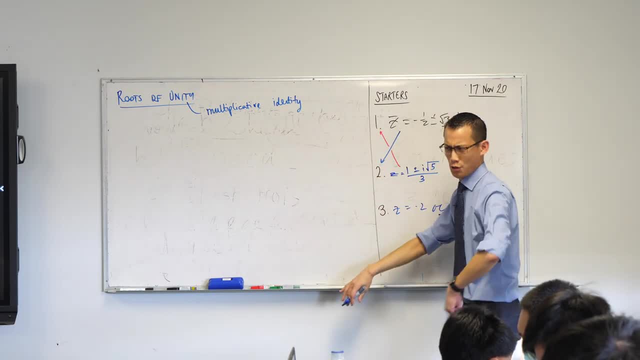 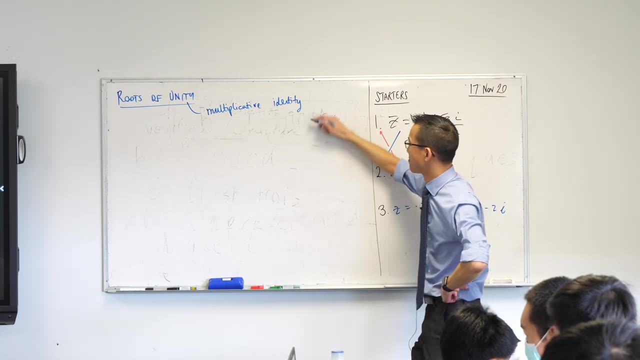 of the course, but it's still interesting anyway. It's called the multiplicative identity. You know, something's a big deal when it's got a big fancy name like that. What is this special hallowed number? And the answer is it's one. You're like, oh really, That was it. Okay, Of course. 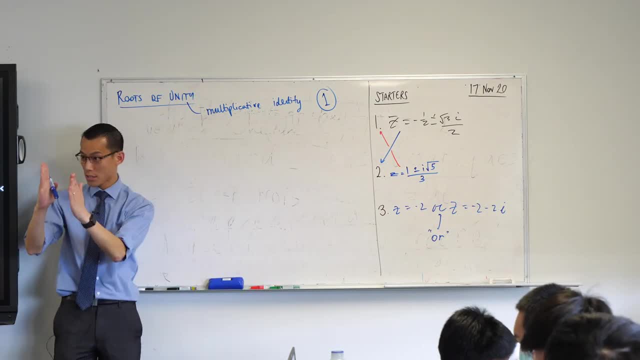 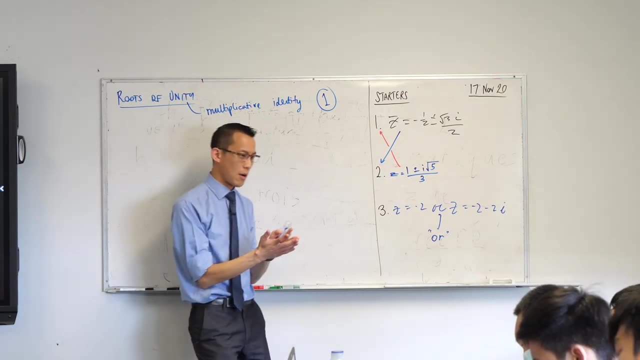 it is one, because that's why it's unity like unit, a single object. And of course it's called the multiplicative identity, because when you multiply something by one, the answer is identical. It doesn't change right Three times. 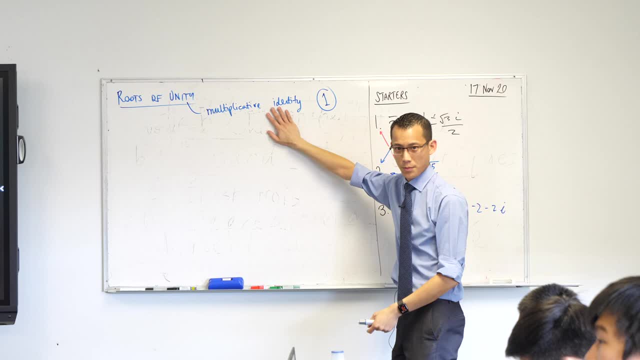 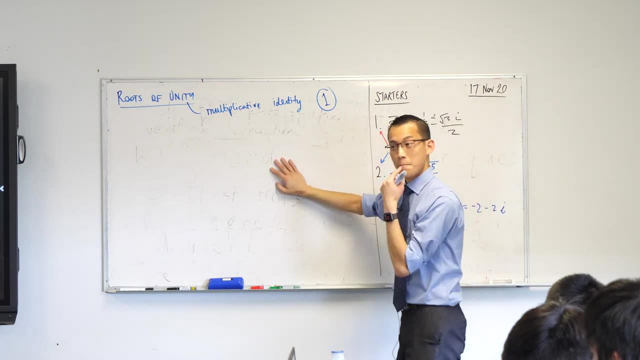 one is three. I times one is I. It doesn't change the number. okay, Now you might think: why is it so special? Like one seems like a very basic number, Why do we get all these special names? For starters, this is not the only number that we give a special name to, right, Like this guy. 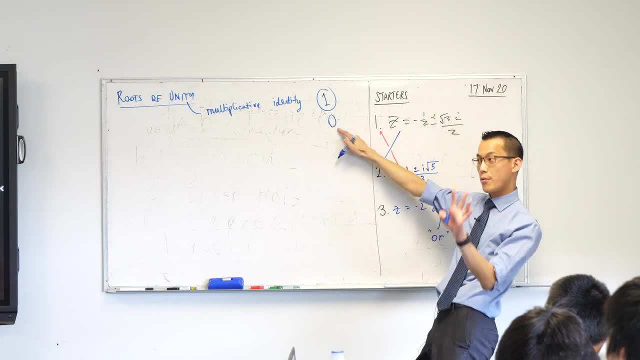 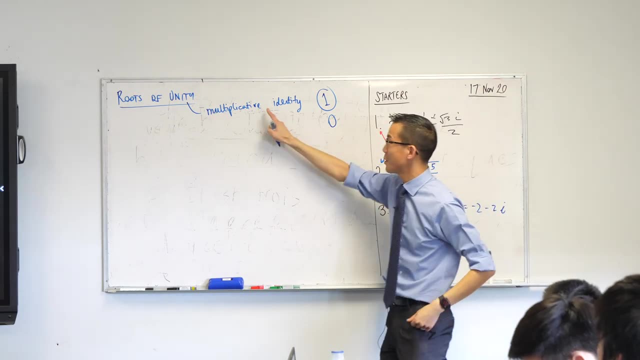 This guy also has a special name, especially when you think about where it is on the complex plane. What do we normally call this number? We call it the origin. It's like ooh special. By the way, it has another name like this as well: It's called the, not the multiplicative. 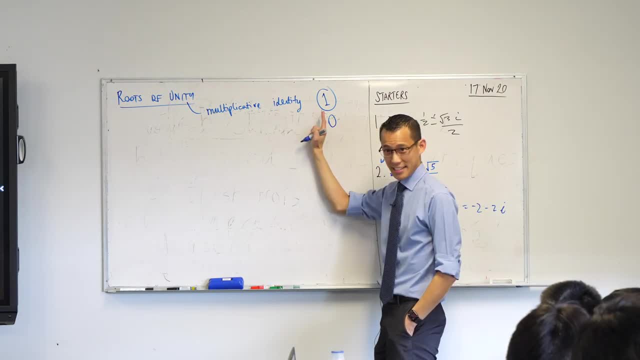 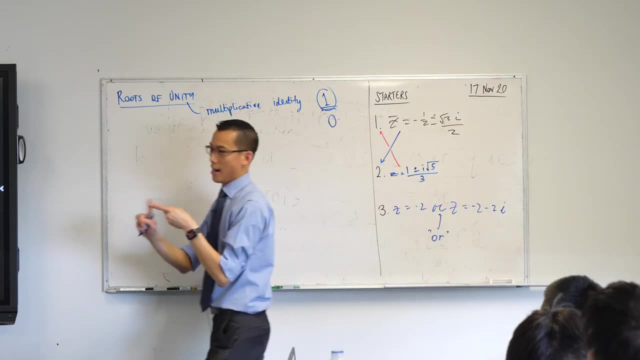 identity. It's called the additive identity because when you add it to things, it doesn't change. It's identical, right? So we want to focus on this number for two reasons. Number one: it's a simple number, So it's easy to deal with, even though we're in complex numbers, okay. So 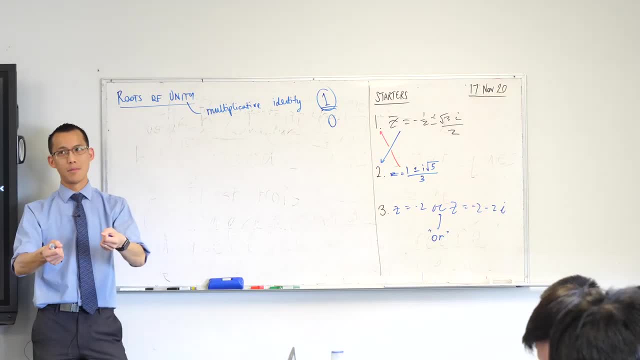 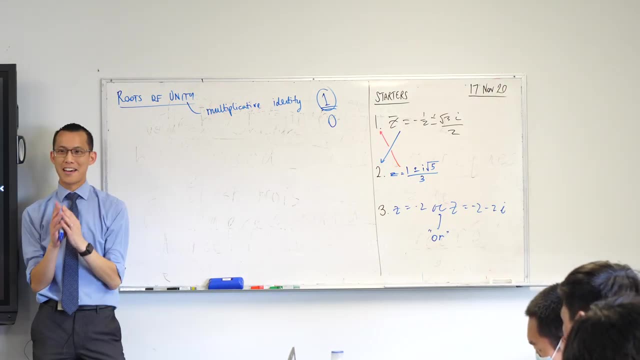 we're going to be able to pull out some algebraic and some other tricks that were useful to us that we can't do with all the rest of the numbers. That's reason number one. Reason number two: the roots of unity actually have some really delicious 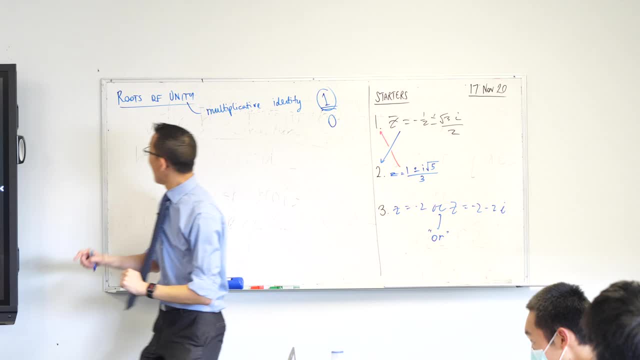 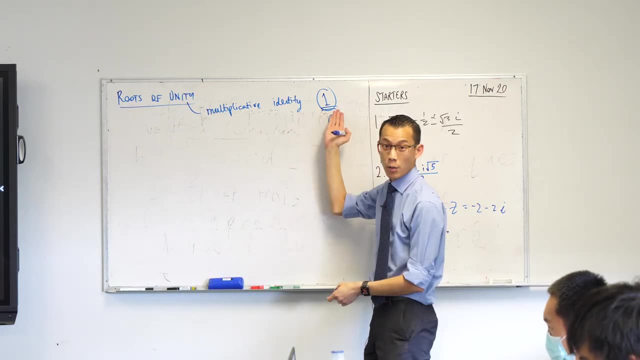 properties, which we'll get to once you find out what they are. okay, So let's start with the first one that we already don't know, which is: we've looked at the square roots of unity. You can work out what they are. by the way, What are the two numbers, the two complex numbers? 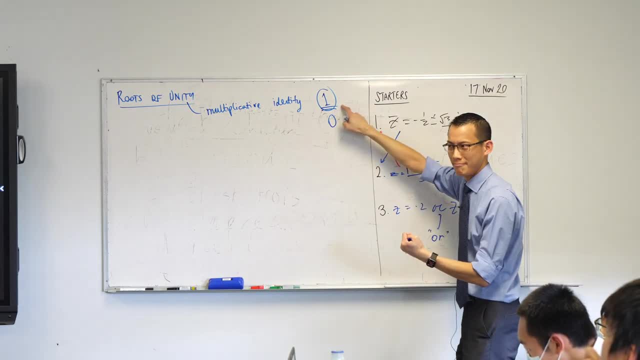 that if you multiply them by themselves will give you one Square roots, Think. I know it's the end of a long day and you might not have much sleep, but you can tell me this: What are the two numbers? Give me at least one of them, I think. think This is just positive one, right? 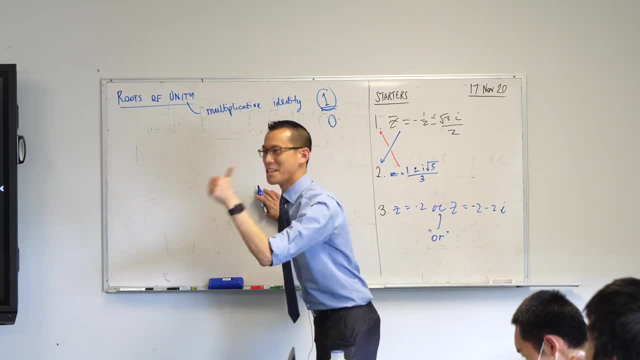 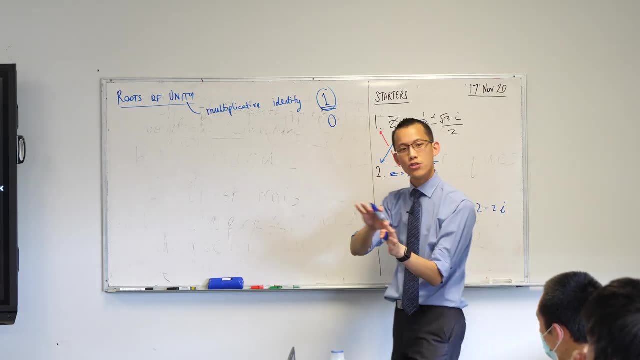 So I'll give you. I'll give you one for free. One is one of the square roots of one, because one times one is one, What's the other one? It's negative one, isn't it right? Now, we usually 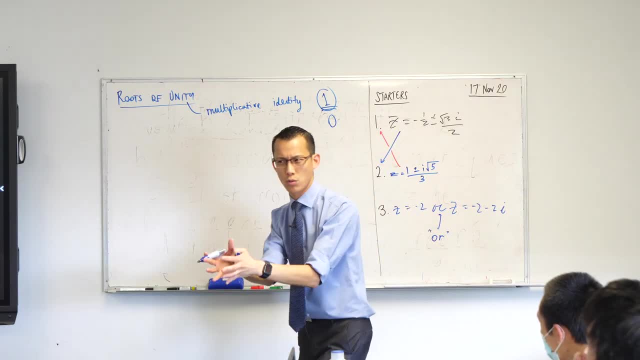 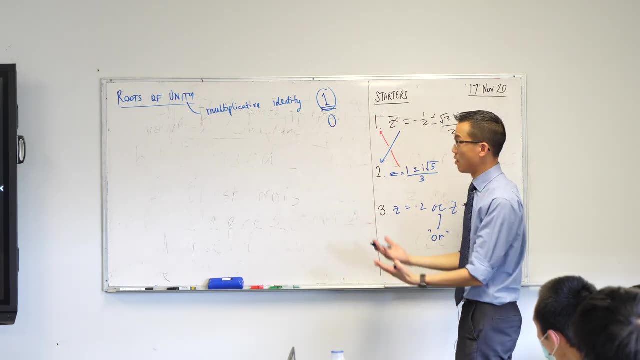 would exclude negative one, because we say the principal square root is just is just one. But actually we've been sort of exploring that negative one times negative one still gives you this. So it is also one of the square roots of unity. The next one is the cube roots of unity. 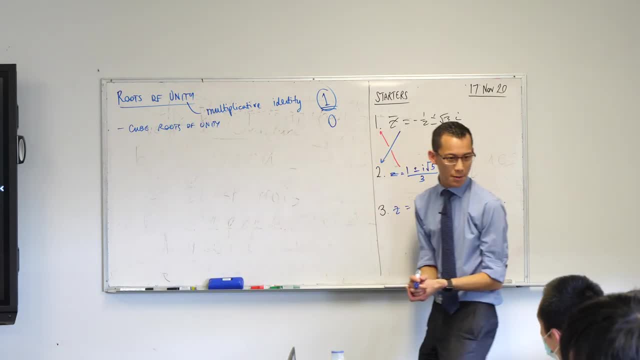 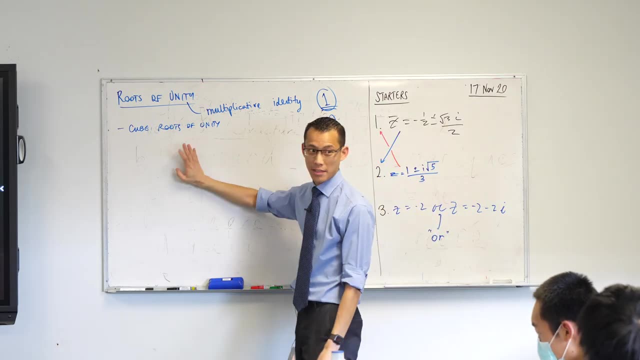 So how do we work out the square roots of unity? Well, we're going to do a little bit of a look at what these cube roots are. Now, the first question I'm going to ask you is: if there are two square roots of every complex number out there, how many cube roots do you expect there to be? 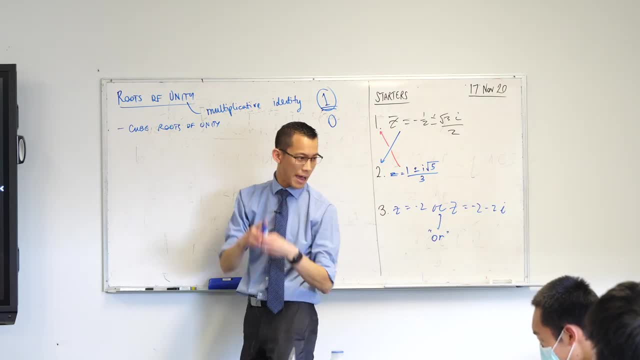 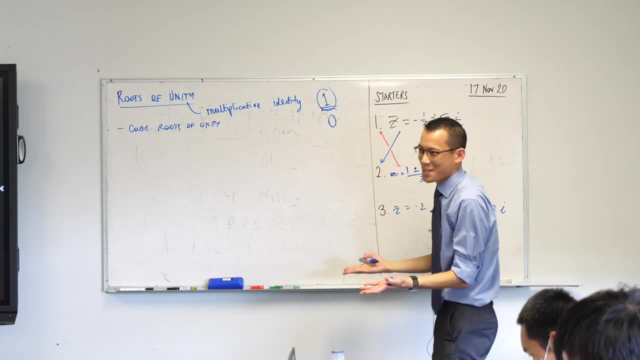 There should be three, right, Like that's the cubing raised to the third power, okay, So how do we find these three? You already know about one of them. It's one, okay. Well, what are the other two? all right. So what we're going to do is we're going to pull out the same kind of trick. 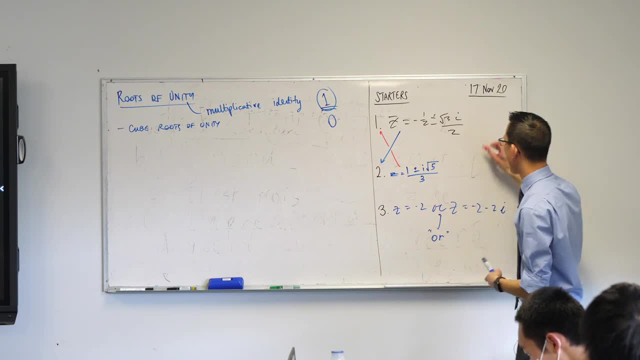 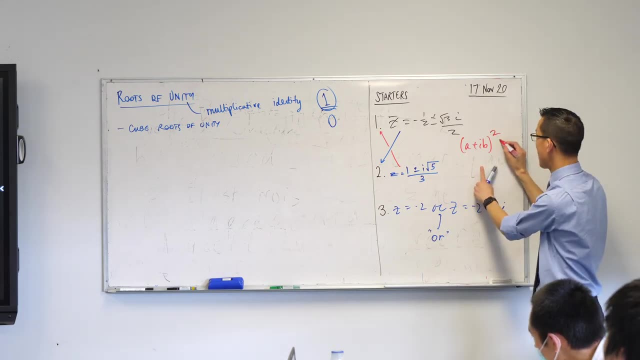 we looked at before. You don't have to write this down, but do you remember when we were finding the square root of a number? we would say, well, there's some number. If you square it, that'll give you whatever complex number you started with right. Well, I'm going to pull. 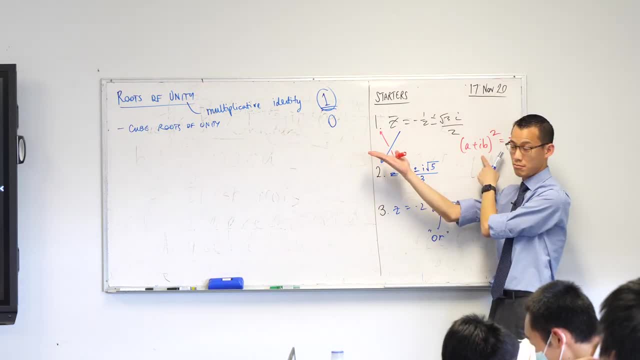 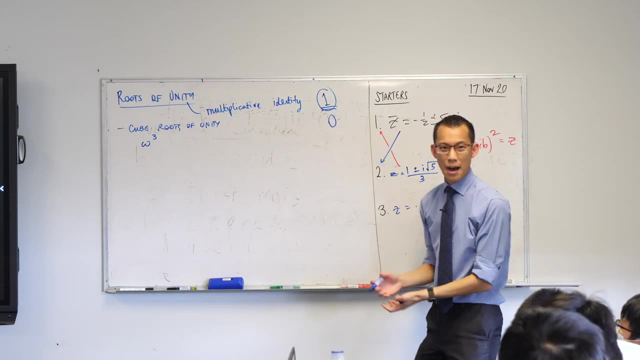 the same trick out, but instead of squaring, I'm going to cube. Okay, let's write this down. So I'm going to use a new Greek letter here. new, This is not a W, it's an omega or a lowercase. 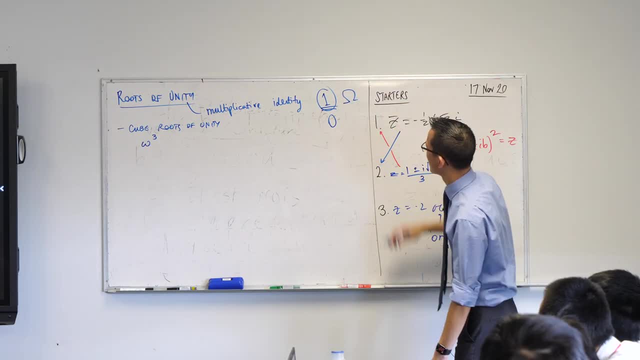 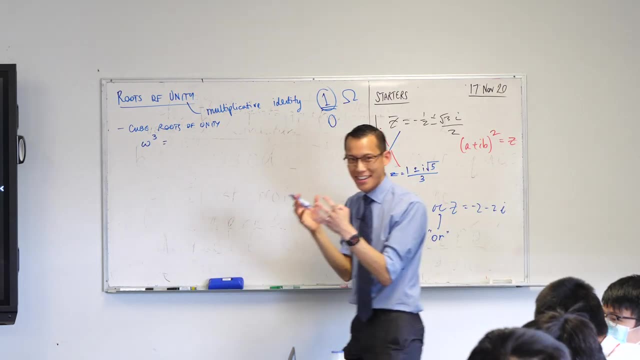 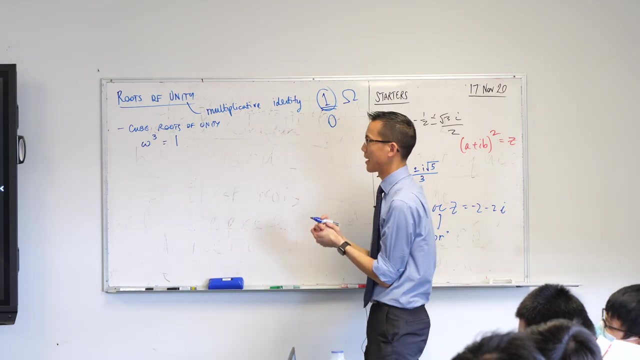 omega. I should say This is the uppercase omega. as fans of Greenland will know, This omega cubed if it's. if this omega is the cube root of unity, then when I cube it, I should end up with one. That's unity, isn't it Okay? and how do I solve this equation? Well, as I mentioned before, 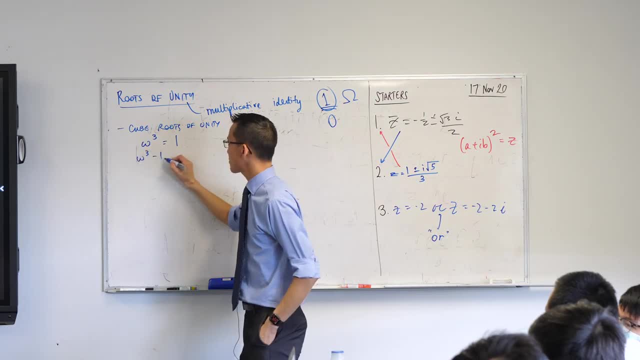 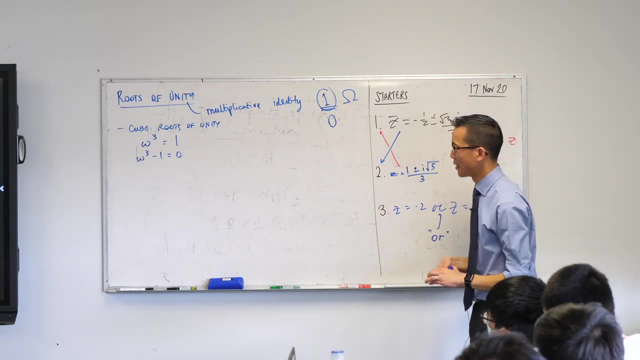 because this is a simple number, I can do some things with it that I can't do with other kinds of numbers. right, I can do some sort of algebraic gymnastics here. okay, Now you guys are used to factorizing things like the sum and difference of squares. We've we know how to do that. 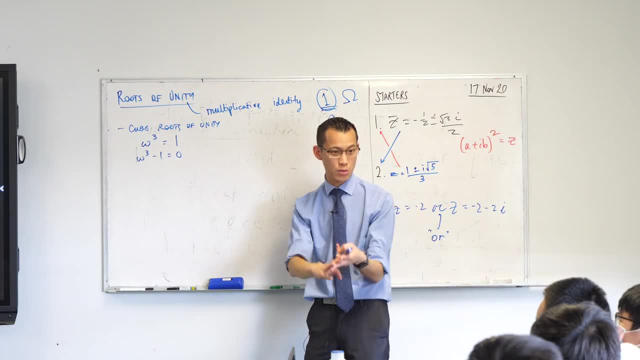 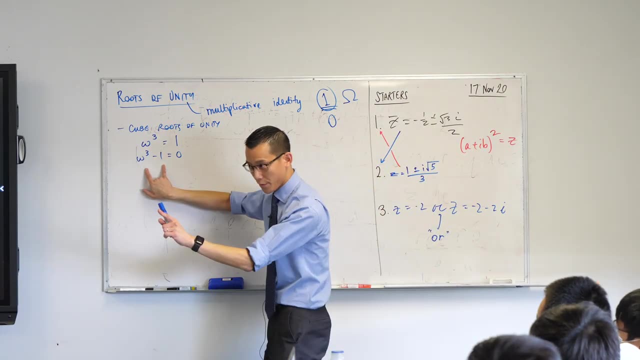 right. We can do difference of squares through normal numbers. We can do sum of squares using the imaginary unit. This is not the sum of difference of squares, it's the sum of difference of cubes. But thankfully for us, there is actually a result that is a nice factorization of this. It 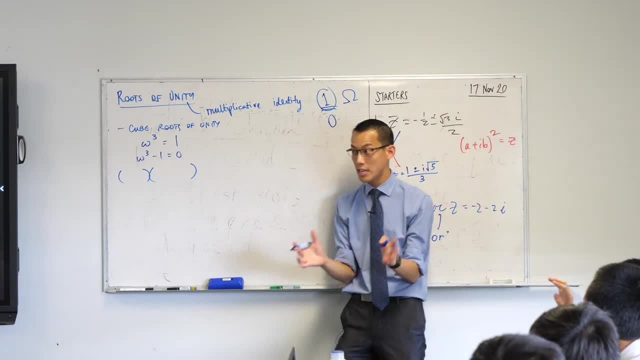 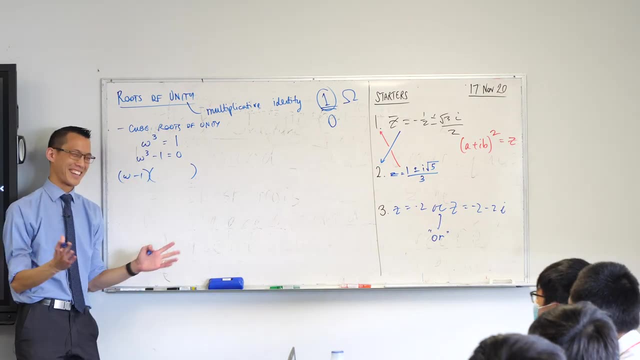 used to be part of the course. it's no longer, but some of you might have encountered it before. Does anyone know what the factorization is, Morgan? So you factorize W minus one, omega minus one- That's okay, I knew what you meant- And then Omega minus one, and then omega. 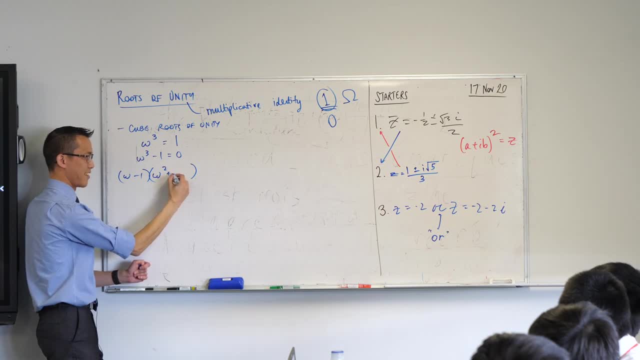 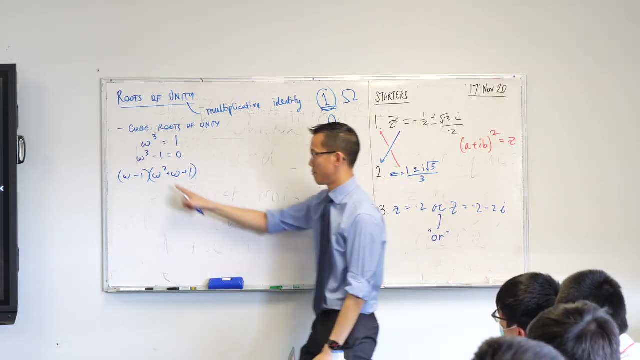 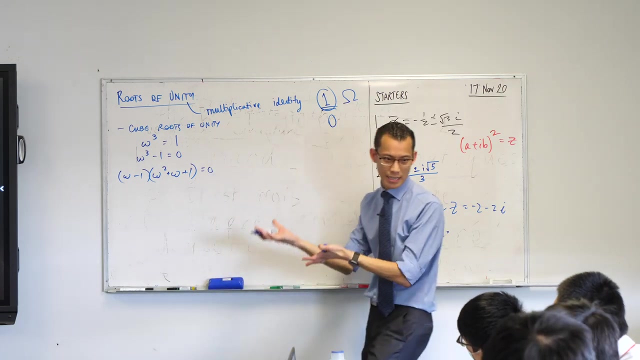 plus one, Yeah, and then omega, and then plus one, Okay. so this, this result right here, is called the difference of cubes. Here's two cubes: you're taking the difference and this is the factorization. As I pointed out, it's not in the course anymore, so don't stress out if you've never. 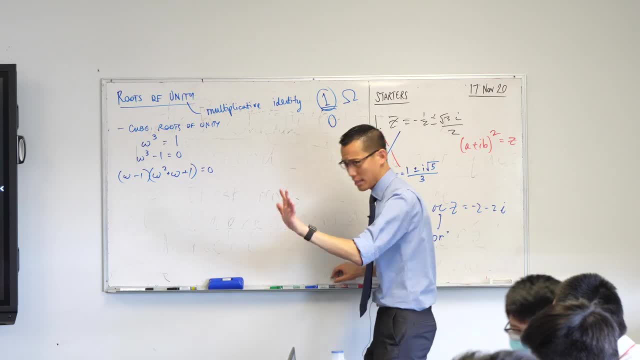 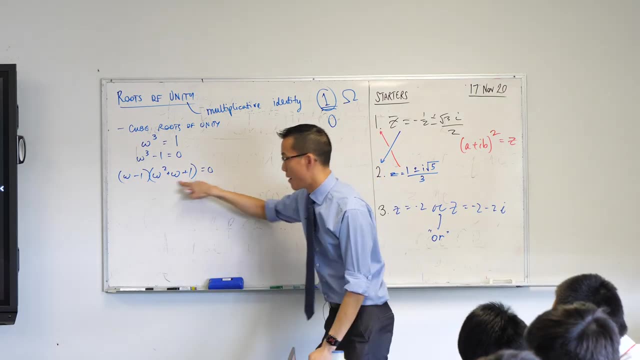 seen this before. But just for the rest of you who are like this is new, let's just content ourselves that this is not just black magic, it actually works. Let's expand it out. it's not hard, right? I'm going to multiply everything by omega and then I'm going to multiply. 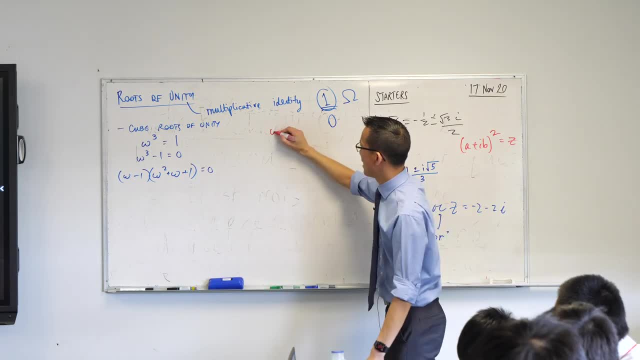 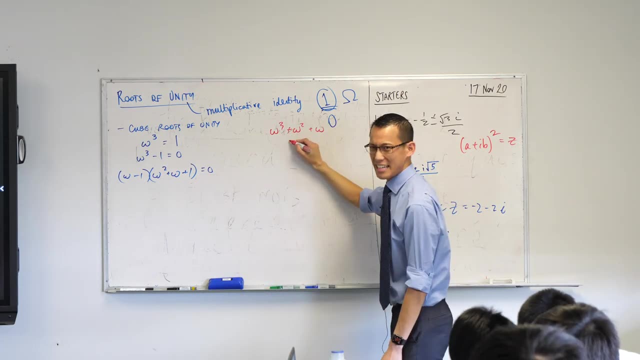 everything by minus one. Watch it just kind of falls out right. Here's me multiplying by omega, and then here's me multiplying by minus one. but I'm just going to write it down here. Are you okay with that? That's the six terms you get. You're like cancel, cancel, cancel. 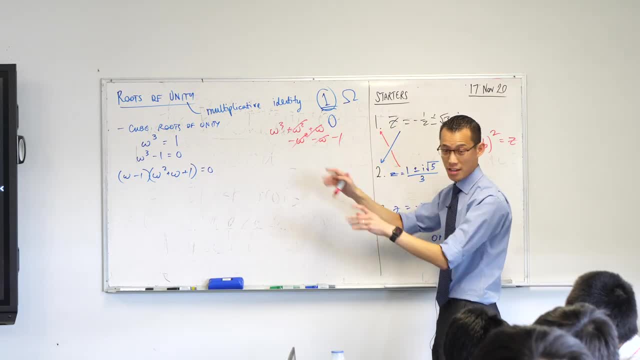 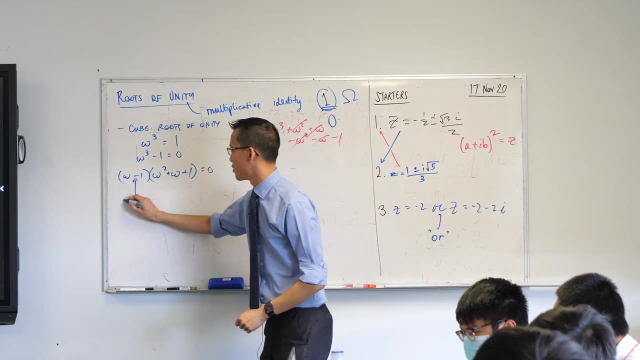 cancel ta-da. there's my difference of cubes. Okay, so it does work. you can content yourself for that. Now, at this point, we're trying to solve for omega. We already knew one of the solutions Here. it is: omega equals One. 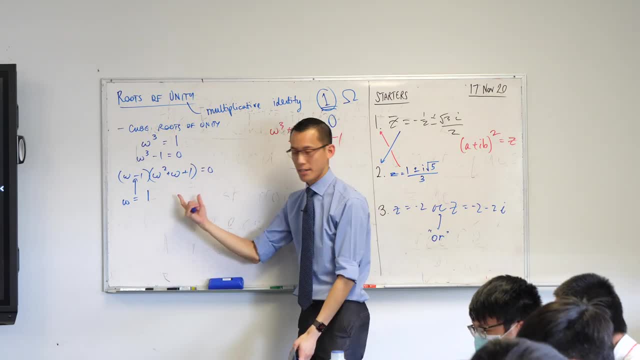 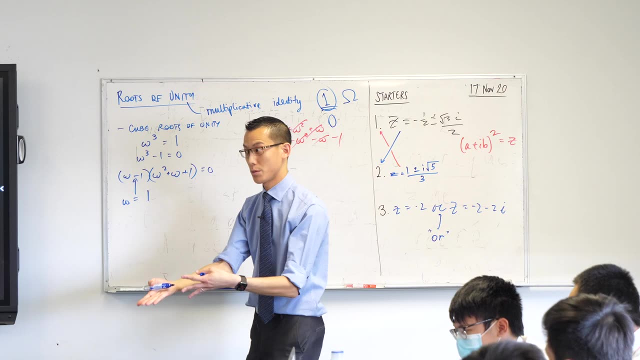 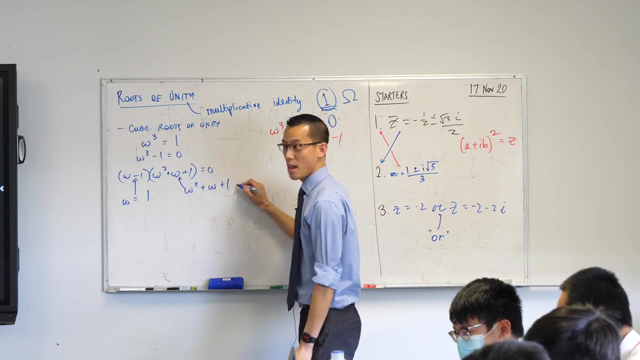 We already knew this. But then you've got this other factor: This can equal zero. we've dealt with that. but if this equals zero, these should be our other mystery: cube roots, right? So I need to solve this guy. Omega squared plus omega plus one equals zero. If I can solve this, I'll have. 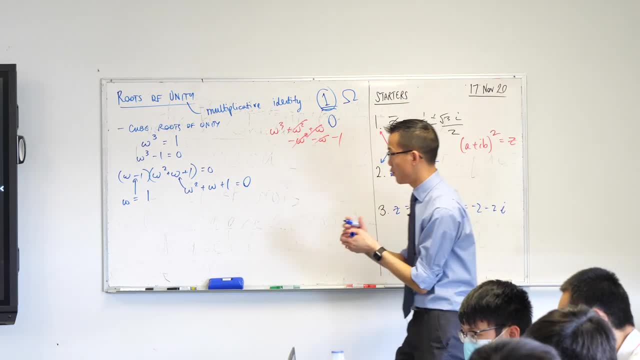 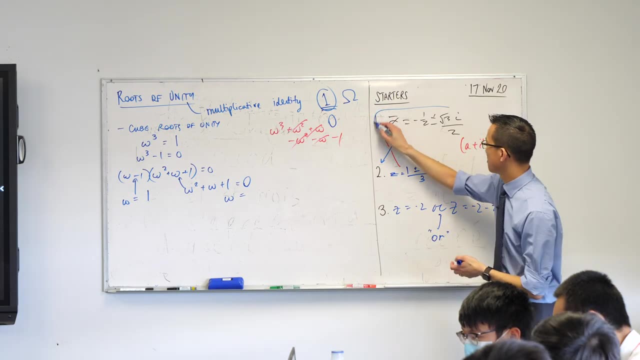 my other two solutions. Now, thankfully for you, you solved this exact equation quite recently, like all of 15 minutes ago. They're right here. These are the other solutions. If you didn't know this, of course, if you didn't have a teacher who gave it to you as a starter question, you'd have to go through. 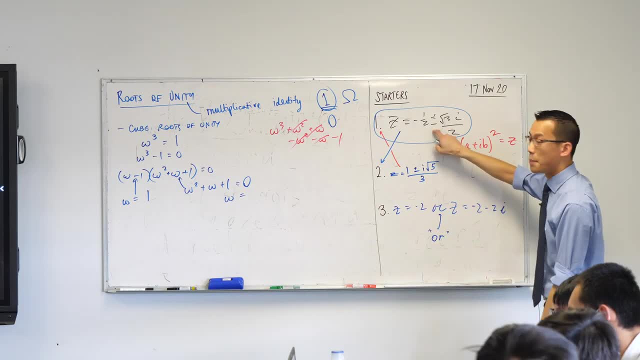 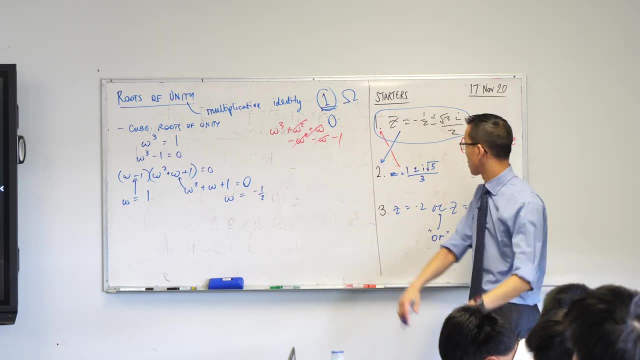 the process of solving this using the quadratic formula. But these would be the answers you get, So let's just quickly jot that down. Negative half. I'm actually going to separate these out as the two separate numbers. I've got the negative case, so minus root three. 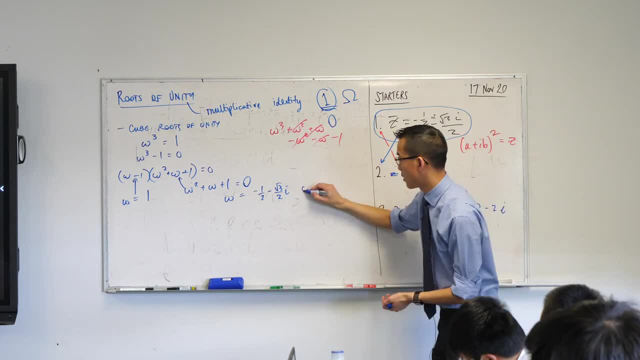 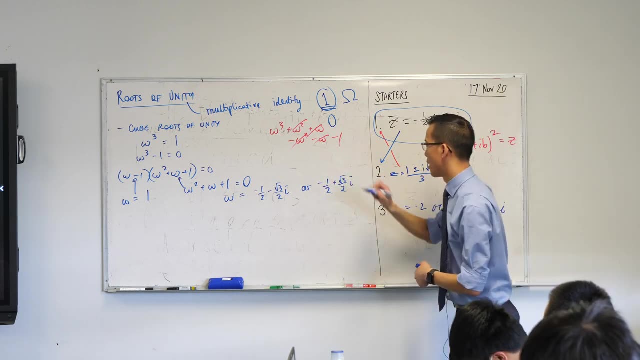 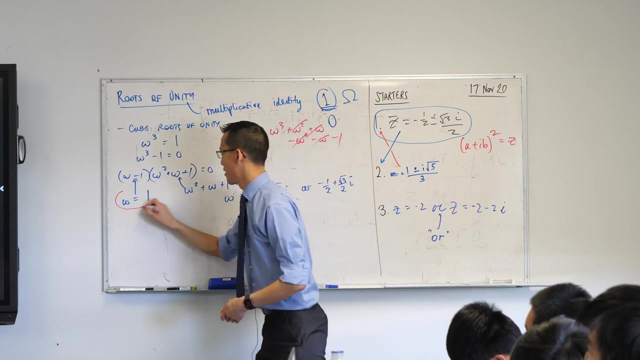 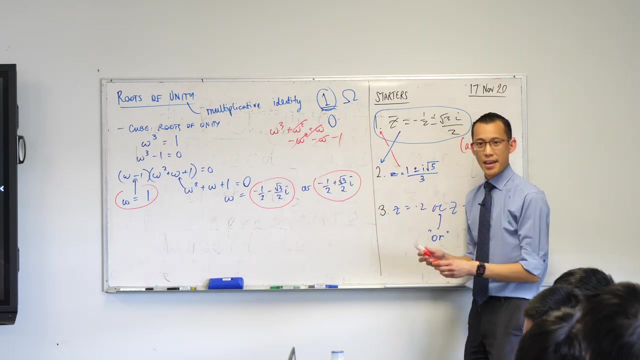 onto i and then I've got the positive case. I've still got negative a half out the front, but now it's plus root three onto i. This is our result. We've got cube roots. We have three numbers. Here's one of them, Here is a second one and here is a third one: Ta-da. 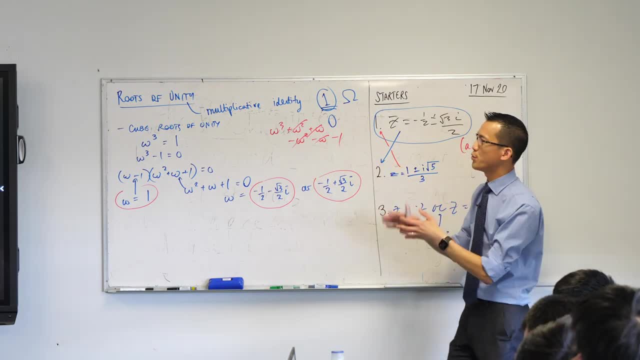 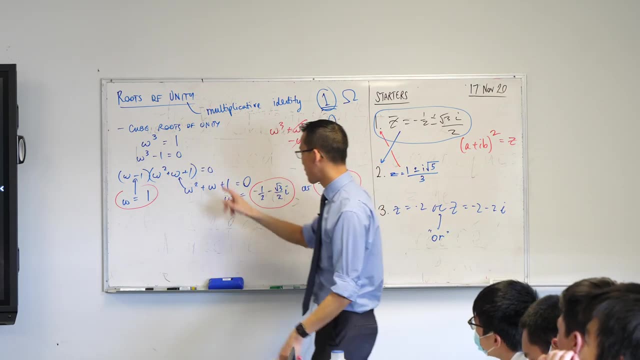 Now what we're going to do is go in two directions from here. I mentioned before that these cube roots have- or actually all the roots of unity have- interesting properties to them. To try and sort of bring that out, what I'd like you to do is to plot on a square root. So 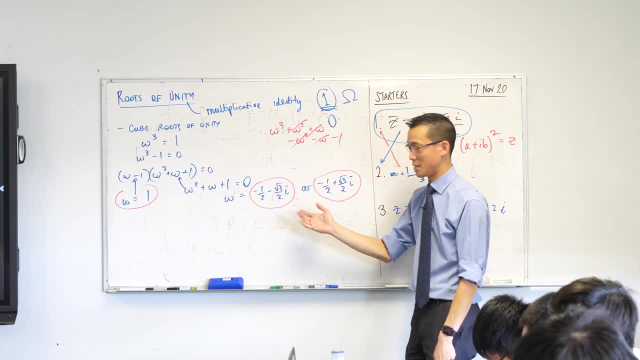 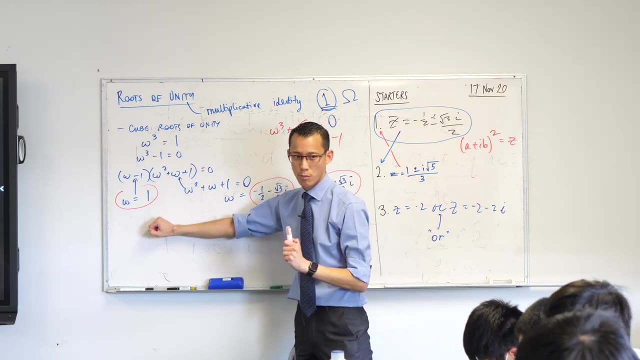 I'm going to plot on an argand diagram all three of these complex numbers. That's the first thing I'm going to ask you to do, And then, secondly, we're going to come up with these same results, but we're going to use a few of the other tools in our toolbox to 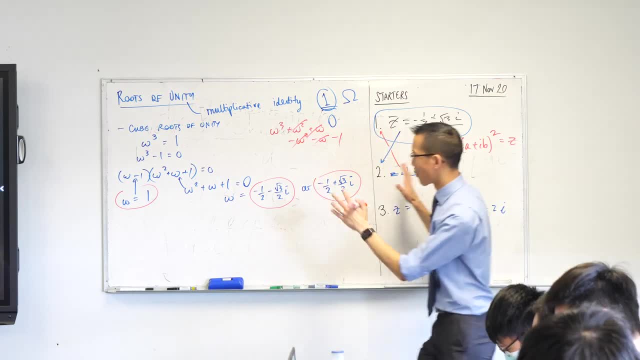 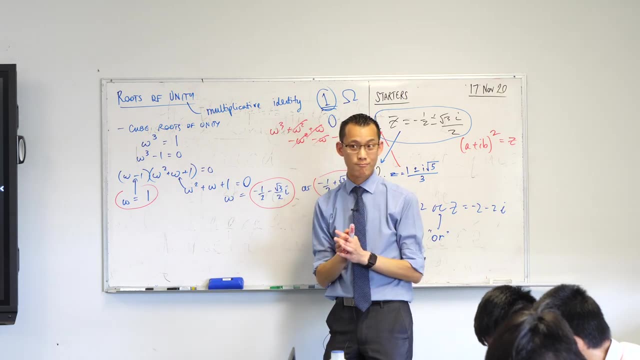 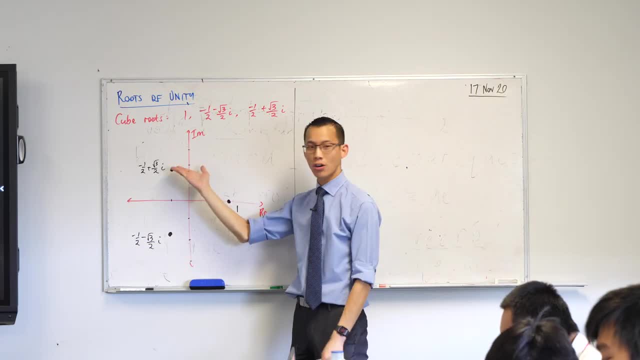 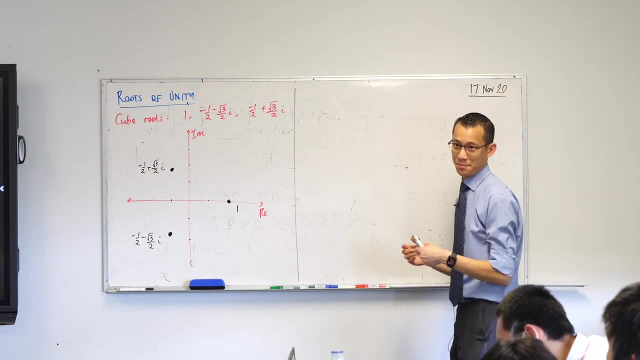 or negative, a half minus root three onto i, and then its conjugate negative, a half plus root three onto i. and there they are positioned. What can you tell me about these particular points on the complex plane? Anyone want to jump out? There's a lot of things. 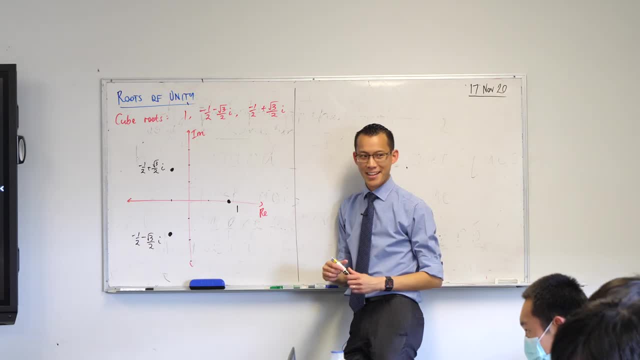 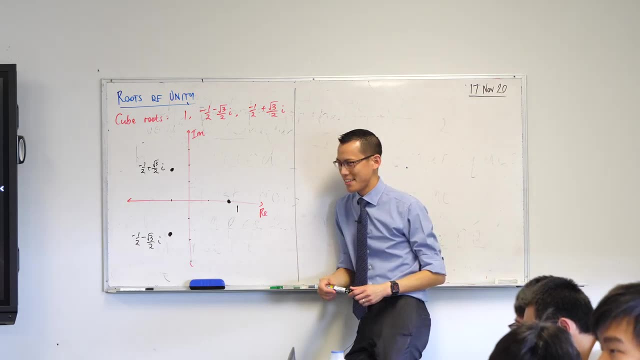 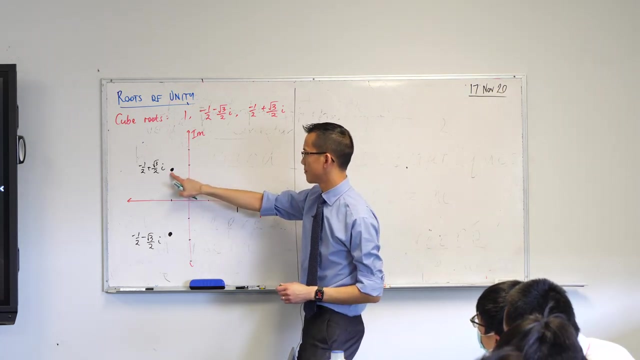 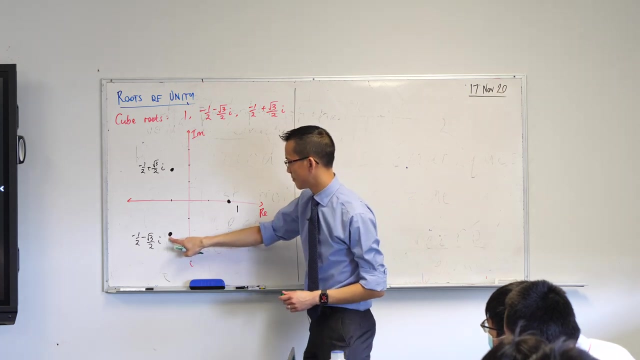 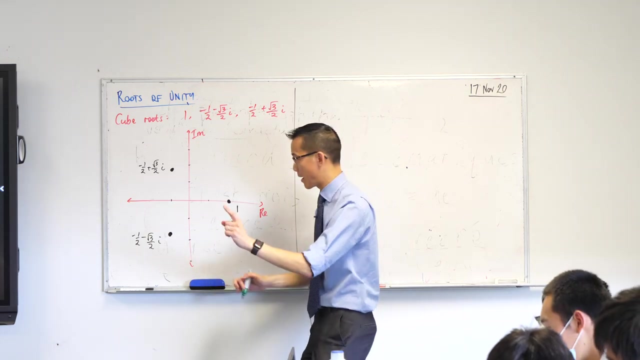 to observe. Anyone want to start us off? Morgan's got a thought. I will hit pause on Morgan, because he's already contributed some great thoughts today. Jiayu, do you notice anything worth pointing out? Ah, okay, So there's some symmetry here, right? We should expect this, because these 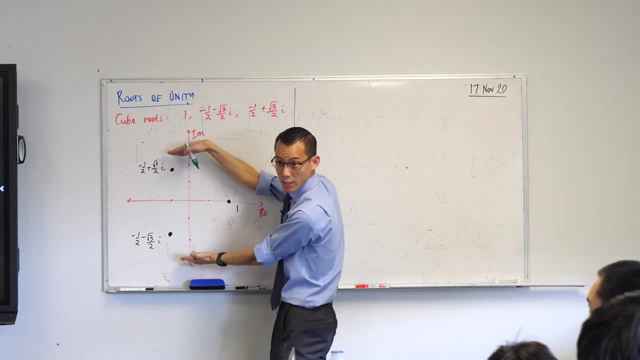 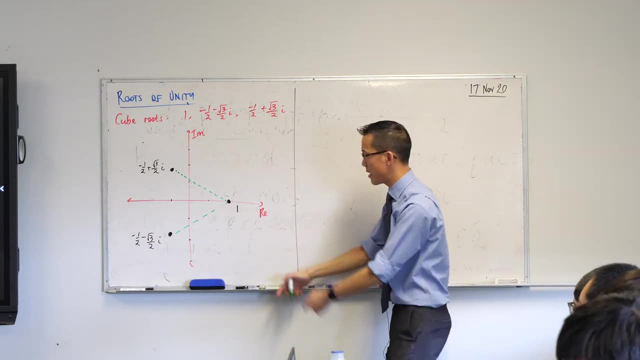 two are conjugates, so they're the exact same distance from the real axis. So the distances that I think Jiayu was talking about were these: Are these the ones you were talking about, right? Right, These two are in fact equal. They're not just equal to each other, they're equal. 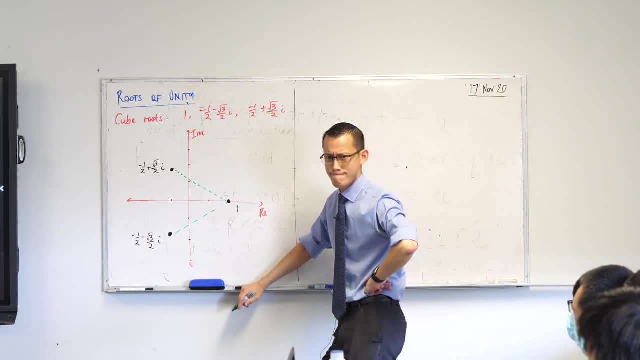 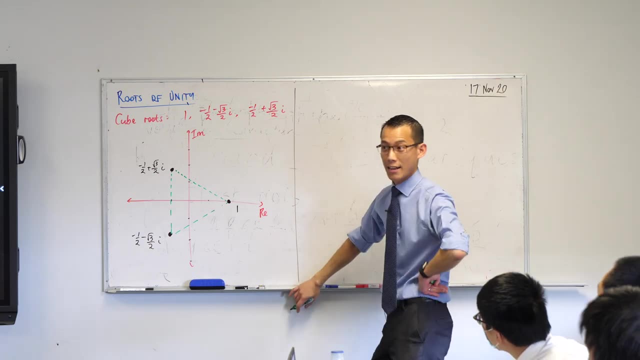 to something else. Where else are they equal to each other? One: Yeah, there's a vertical between these two conjugates, right? In fact, this sure looks like an equilateral triangle. Now I should point out, it looks equilateral I. 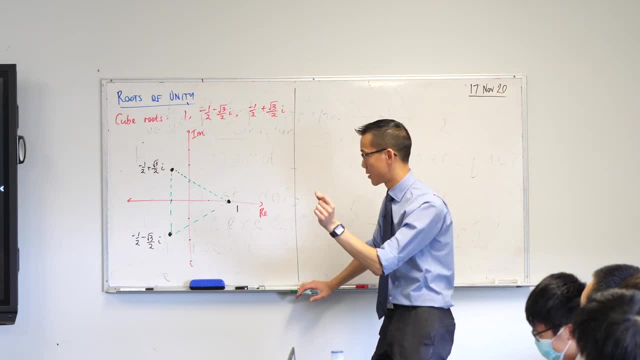 don't know if your diagram is good enough to reason that, but we can actually prove it Before we do that. are there any other things like, apart from the fact that it looks equilateral, any other things that we can observe? Right?